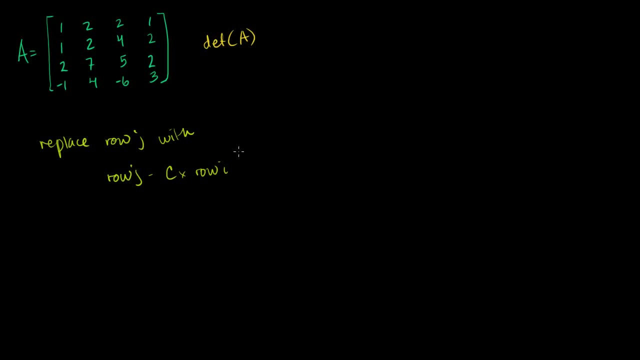 Times row i: it does not change the determinant of A. We saw that I think it was two videos ago, So this was a pretty big realization. We can do these type of row operations and it won't change the determinant. 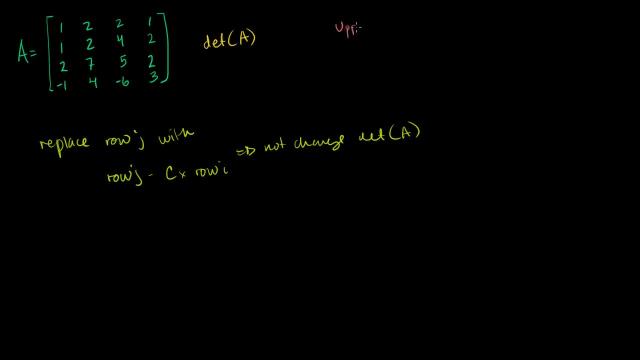 The other realization we had was that these upper triangular matrices, you can figure out their determinant. So what is upper triangular? Let me just review it. The upper triangular everything below the diagonal. so let's say the diagonal has- let me just draw its terms, like: 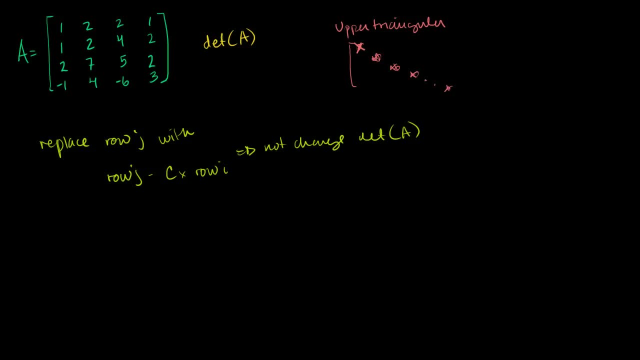 that these are some non-zero terms, or they don't have to be. then, upper triangular, everything below the diagonal is a 0, and everything above the diagonal probably isn't a 0,, but you never know. but they're non-zero terms. 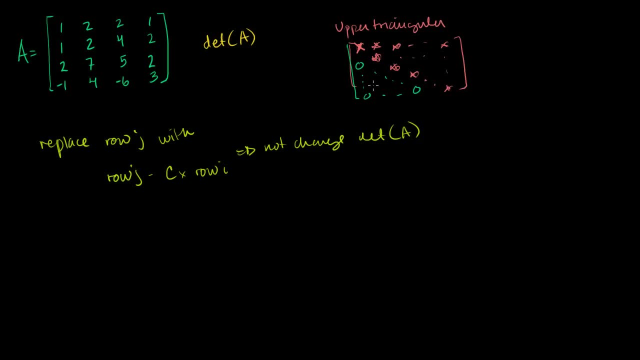 So all the red stuff here is non-zero. all the stuff in green is 0.. I didn't touch on it in that video, but there is also such a thing as a lower triangular that you might have guessed how it looks. Everything above the main diagonal is 0, so this is the 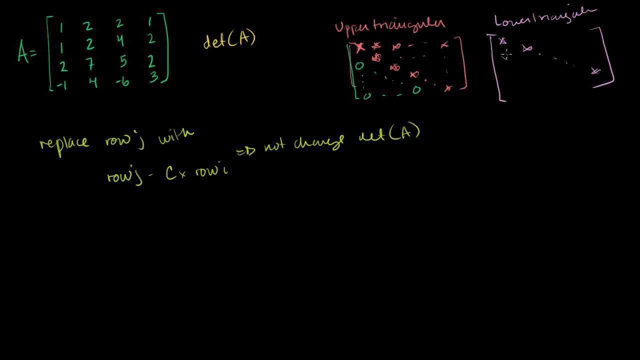 main diagonal right here all the way down. like that, All of these guys are going to be non-zero, all of that's going to be non-zero, and then the 0's are going to be above the diagonal, like that. We saw in the last video that the determinant of this 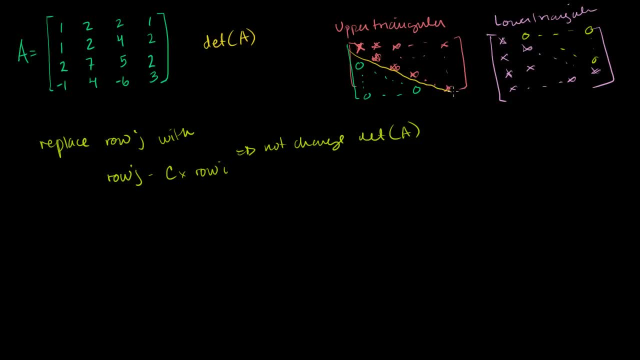 guy is just equal to the product of the diagonal entries, which is a very good or it's a very simple way of finding a determinant, And you could use the same argument we made in the last video to say that the same is true of the lower triangular. 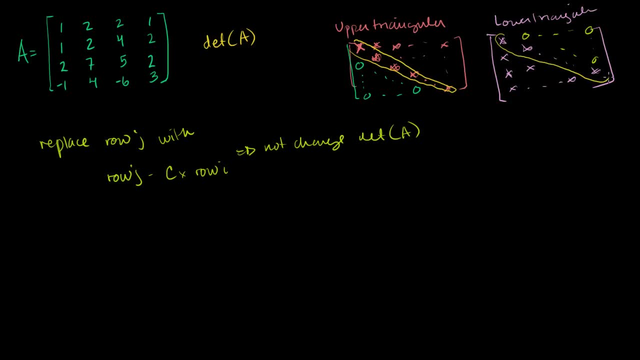 matrix, that its determinant is also just the product of those entries. I won't prove it here, but you can use the exact same argument you used in the video that I just did on the upper triangular. So, given this, that the determinant of this is just. 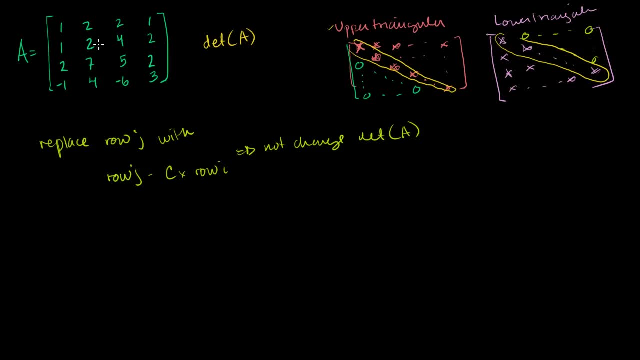 the product of those guys and that I can perform row operations on this guy And not change the determinant. Maybe a simpler way to calculate this determinant is to get this guy into an upper triangular form and then just multiply the entries down the diagonal. 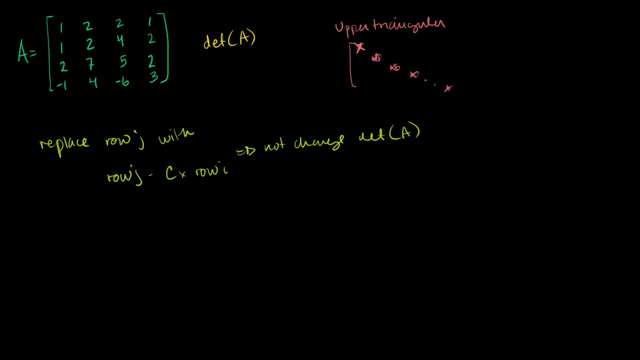 that these are some non-zero terms, or they don't have to be. then, upper triangular: everything below the diagonal is a 0.. Everything below the diagonal is a 0, and everything above the diagonal probably isn't a 0,, but you never know. but 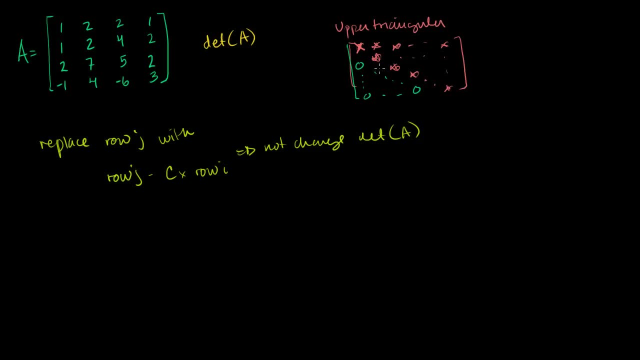 they're non-zero terms. So all the red stuff here is non-zero. all the stuff in green is 0.. I didn't touch on it in that video, but there is also such a thing as a lower triangular that you might have guessed. 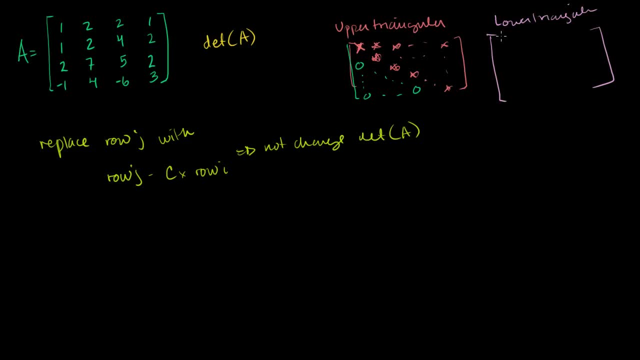 how it looks. Everything above the main diagonal is 0, so this is the main diagonal right here, all the way down, like that, All of these guys are going to be non-zero, all of that's going to be non-zero, and then the 0's are going to be above. 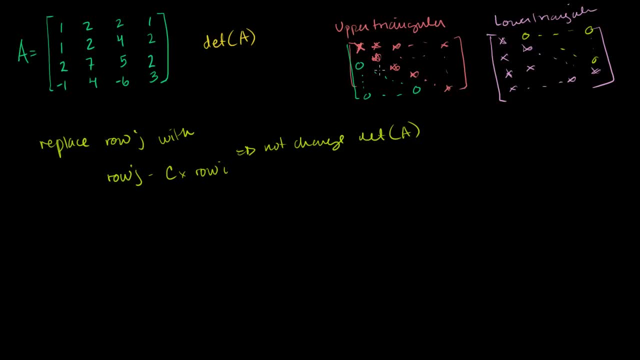 the diagonal like that. We saw in the last video that the determinant of this guy is just equal to the product of the diagonal entries, which is a very simple way of finding a determinant, And you could use the same argument we made in the last. 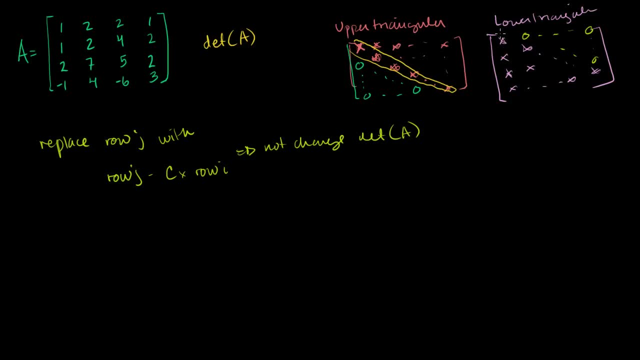 video to say that the same is true of the lower triangular matrix, that its determinant is also just the product of those entries. I won't prove it here, but you can use the exact same argument you used in the video that I just did on the upper. 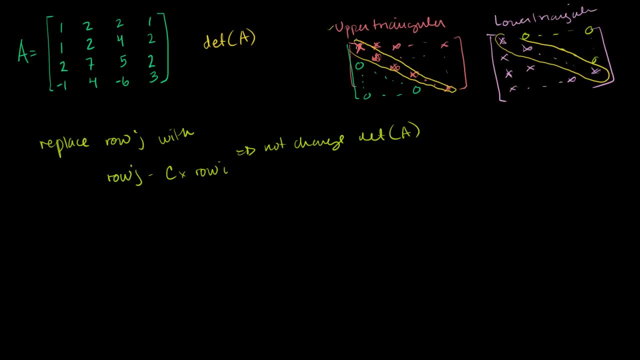 triangular. So, given this, that the determinant of this is just the product of those guys and that I can perform row operations on this guy And not change the determinant, Maybe a simpler way to calculate this determinant is to get this guy into an upper triangular form and then just 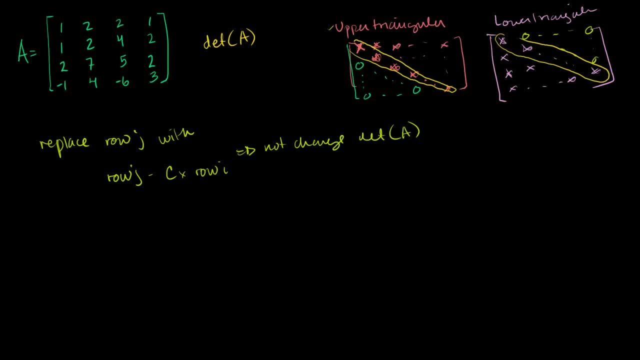 multiply the entries down the diagonal. So let's do that. So we want to find the determinant of A. So the determinant of A, let me rewrite A right here. It's 1, 2,, 2, 1.. 1, 1, 2, 4, 2, 2, 7, 5, 6, 7,, 8,, 9,, 10,, 11,, 12,, 13,, 14,, 15,, 16,. 17,, 18,, 19,, 20,, 21,, 22,, 23,, 24,, 25,, 26,, 27,, 28,, 29,, 30,, 31,, 32,, 33,, 34,, 35,, 34,, 35,, 36,, 37,, 38,, 39,, 40,, 41,, 42,, 43,, 42,, 43,, 44,, 44,, 45,. 45,, 46,, 47,, 48,, 39,, 42,, 44,, 45,, 48,, 49,, 41,, 42,, 43,, 43,, 42,, 45,, 46,. 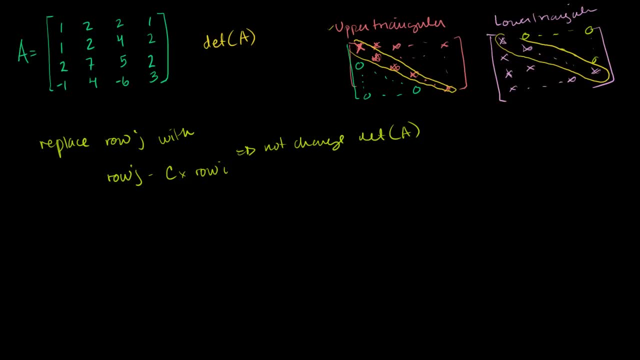 So let's do that. So we want to find the determinant of A. So the determinant of A, let me rewrite A right here. It's 1, 2, 2, 1.. 1, 1, 2, 4, 2, 2, 7, 5, 6, 7, 8, 9, 10,, 11,, 12,, 13,, 14,, 15,, 16,. 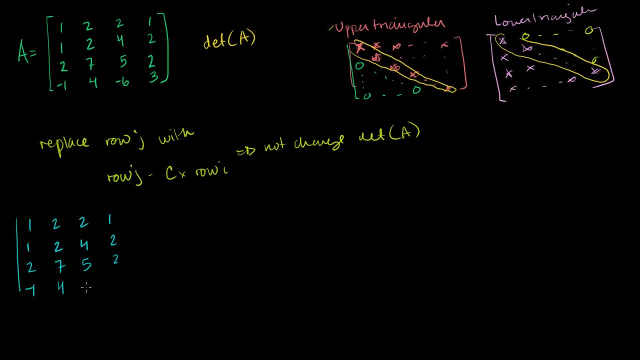 17,, 18,, 19,, 20,, 21,, 22,, 23,, 24,, 25,, 26,, 27,, 28,, 29,, 30,, 31,, 32,, 33,, 34,, 35,, 36,, 37,, 38,, 39,, 40,, 42,, 44,, 45,, 46,, 47,, 48,, 41,, 42,, 42,. 45,, 46,, 47,, 48,, 42,, 42,, 43,, 44,, 45,, 46,, 47,, 49,, 49,, 50,, 51,, 52,, 51,, 52,, 52,. 53,, 53,, 53,, 53,, 54,, 55,, 56,, 57,, 52,, 54,, 56,, 57,, 58,, 58,, 79,, 80,, 80.. 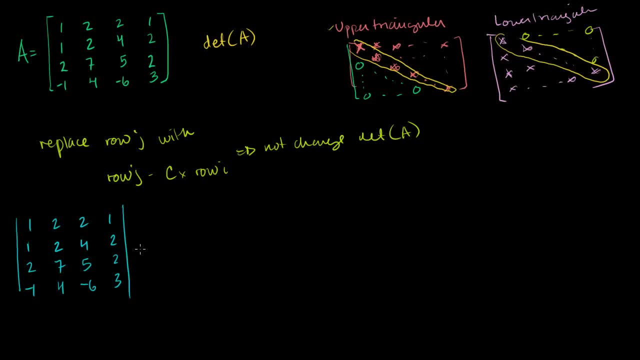 Now let's put this in. let's try to get this into upper triangular form. So let's replace the second row with the second. So I'm just going to keep the first row the same: 1, 2,, 2, 1.. 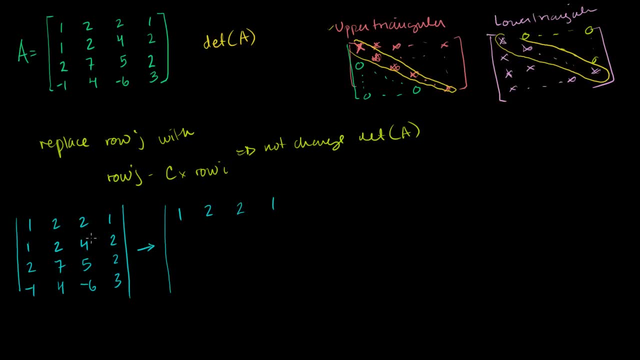 And let's replace the second row with the second row minus the first row. The second row minus the first row is going to be equal to 1 minus 1 is 0.. So in this case the constant is just 1.. So 1 minus 1 is 0.. 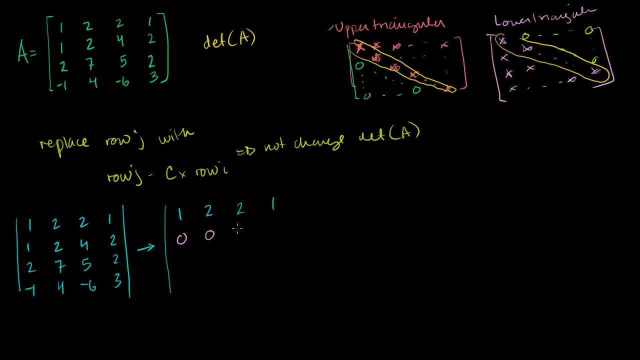 2 minus 2 is 0.. 4 minus 2 is 2.. 2 minus 1 is 1.. Now let's replace the third row with the third row minus 2 times the second row. So 2 minus 2 times 1 is 0.. 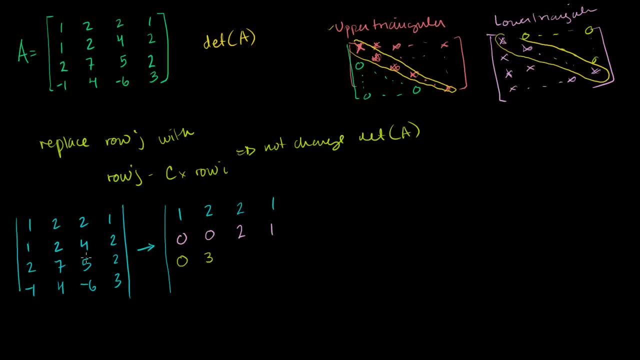 7 minus 2 times 2 is 3.. 5 minus 2 times 2 is 1.. 2 minus 2 times 1 is 0.. And then let's get a good color here, do pink. Let's replace the last row with the last row, essentially. 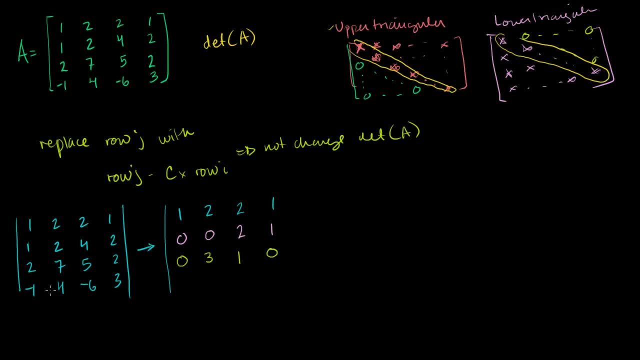 plus the first row. You could say minus, minus 1 times the first row, which is the same thing as the last row Plus the first row. So minus 1 plus 1 is 0.. 4 plus 2 is 6.. 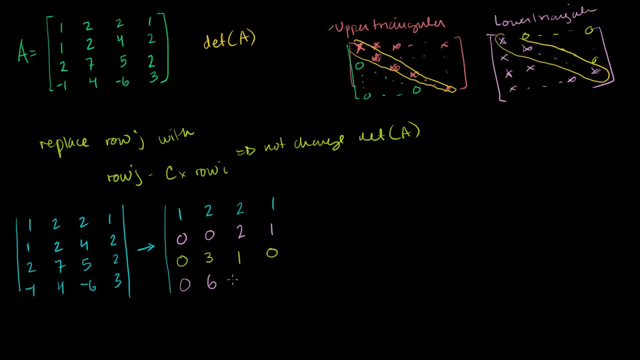 Minus 6 plus 2 is minus 4.. And then 3 plus 1 is 4.. So there we have it like that, And this guy has two 0's here, so maybe I want to swap some rows. So let me swap some rows. 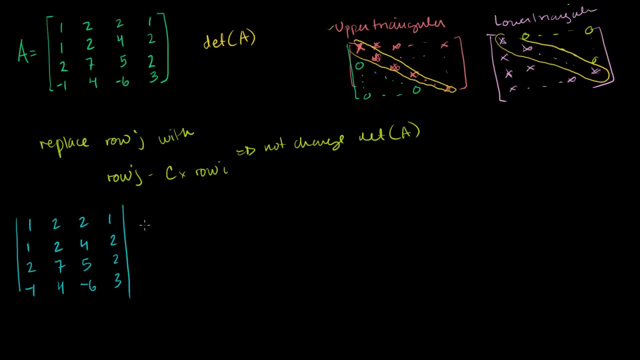 Now let's put this in, let's try to get this into upper triangular form. So if we let's replace the second row with the second, So I'm just going to keep the first row the same: 1, 2,, 2, 1.. 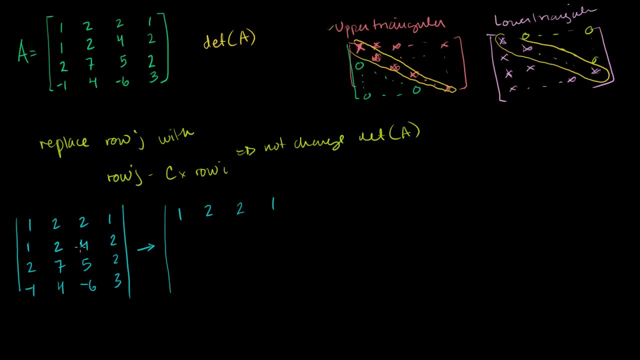 And let's replace the second row with the second row minus the first row. The second row minus the first row is going to be equal to 1.. to 1 minus 1 is 0.. So in this case, the constant is just 1.. 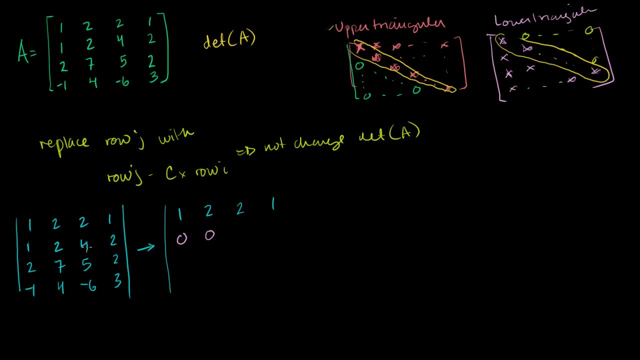 So 1 minus 1 is 0.. 2 minus 2 is 0.. 4 minus 2 is 2.. 2 minus 1 is 1.. Now let's replace the third row with the third row, minus 2 times the second row. 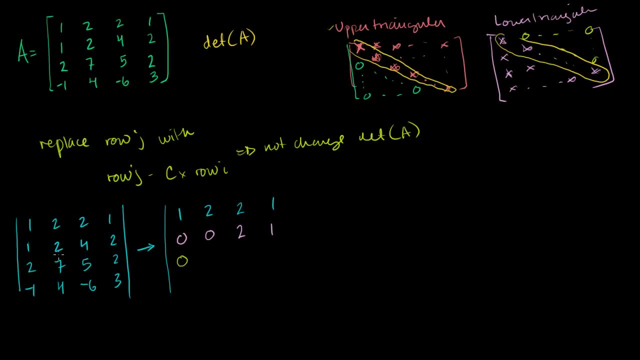 So 2 minus 2 times 1 is 0.. 7 minus 2 times 2 is 3.. 5 minus 2 times 2 is 1.. 2 minus 2 times 1 is 0.. And then let's get a good color here, do pink? 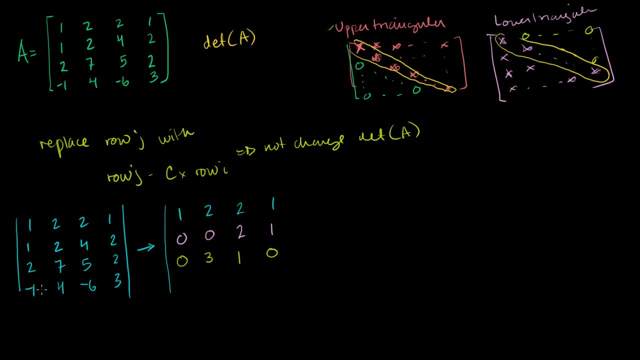 Let's replace the last row with the last row, essentially plus the first row. You could say: minus minus 1 times the first row is the same thing as the last row plus the first row. So minus 1 plus 1 is 0.. 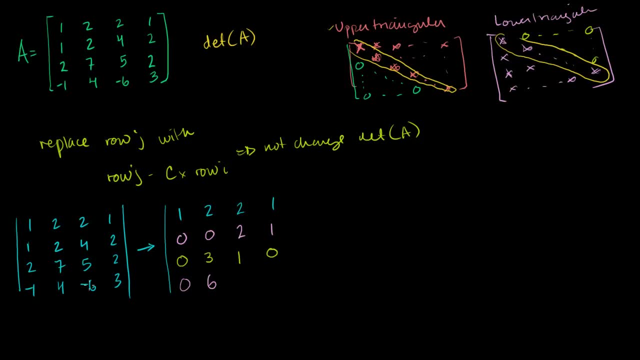 4 plus 2 is 6.. Minus 6 plus 2 is minus 4.. And then 3 plus 1 is 4.. So there we have it like that, And this guy has two 0's here, so maybe I. 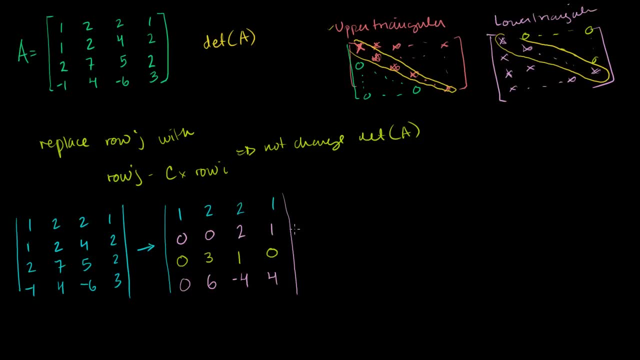 want to swap some rows, So let me swap some rows. If we swap rows, what happens? So let me swap the middle two rows, just for fun. Well, not just for fun, Because I want a middle two. I want a pivot entry right here. 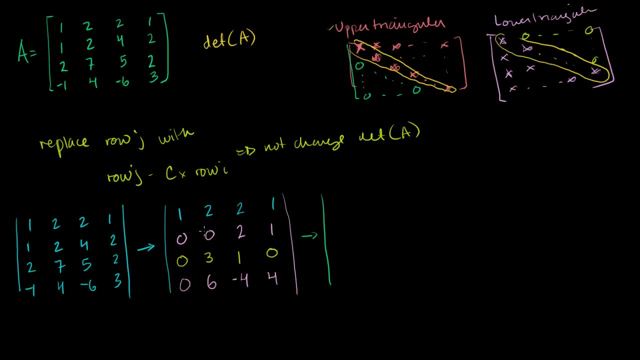 Or I shouldn't say pivot entry. I want to do it in upper triangular form, So I want a non-zero entry here. This is a 0, so I'm going to move this guy down, So I'm going to keep the top row the same. 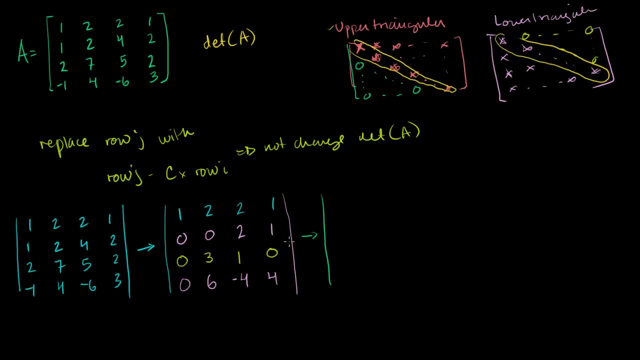 If we swap rows, what happens? I'm going to swap the middle row. I'm going to swap the middle two rows, just for fun. Well, not just for fun, Because I want a pivot entry right here, Or I shouldn't say pivot entry. 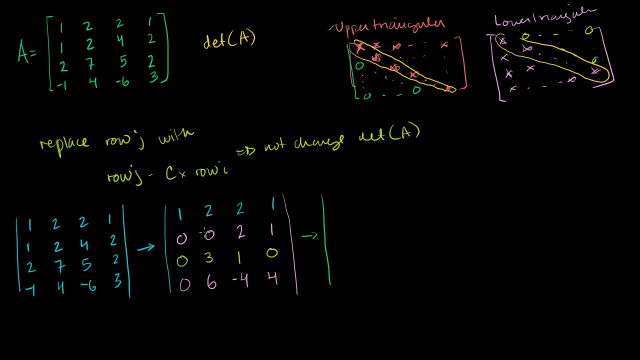 I want to do it in upper triangular form, So I want a non-zero entry here. This is a 0, so I'm going to move this guy down. So I'm going to keep the top row the same: 1, 2,, 2, 1.. 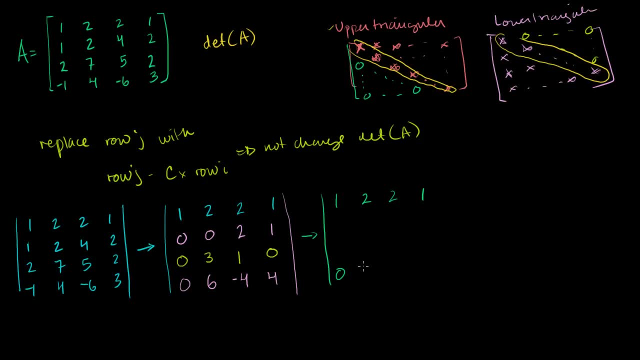 I'm going to keep the bottom row the same: 0, 0, 6, minus 4, 4.. And I'm going to swap these guys right here. So this is going to be 0, 3, 1, 0.. 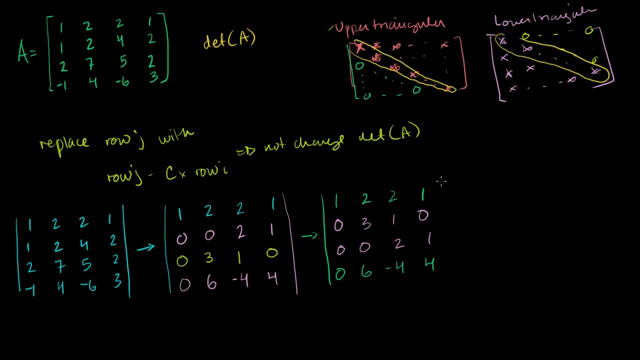 And then 0,, 0,, 2,, 1.. Now can I just swap entries like that? Well, I can, but you have to remember that when you swap entries, your resulting determinant is going to be the negative of your original determinant. 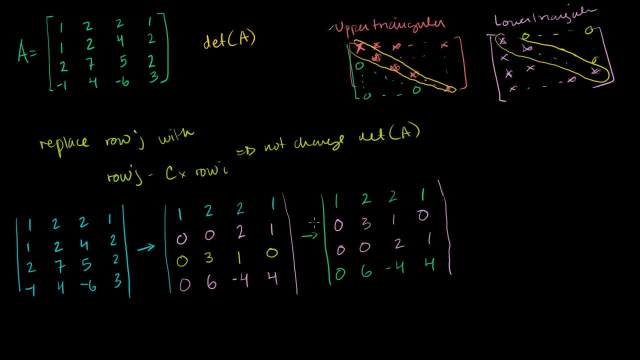 So if we swap these two guys, the determinant of this is going to be the negative of this determinant. When you swap two rows, you just flip the sign of the determinant. We saw that That was one of the first videos we did on these kind of. 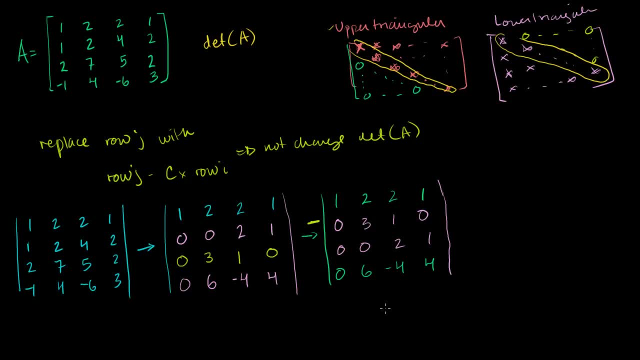 messing with the determinants. Now, what do we want to do here? To get this guy into upper triangular form. it'd be nice to get this to be a 0. So to get that to be a 0,, let me keep. 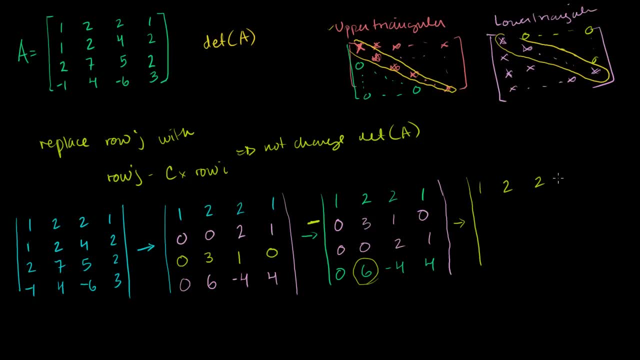 everything else the same. So I have a 1, 2,, 2, 1.. I have a 0, 3,, 1, 0.. The third row is 0, 0,, 2, 1.. 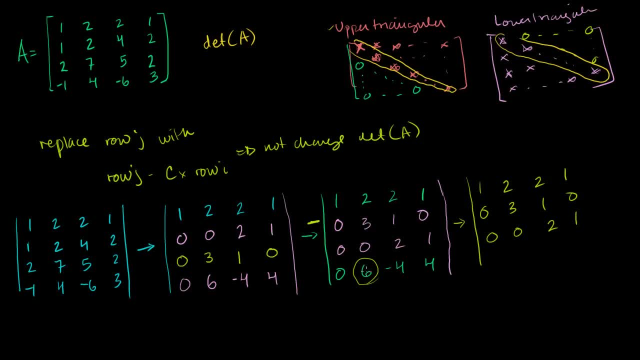 And now this last row. let me replace it with the last row, minus 3 times this row. So let me write this. I'll write it like this: Well, I have to carry that negative sign as well. So I'm going to replace this last row with the last row. 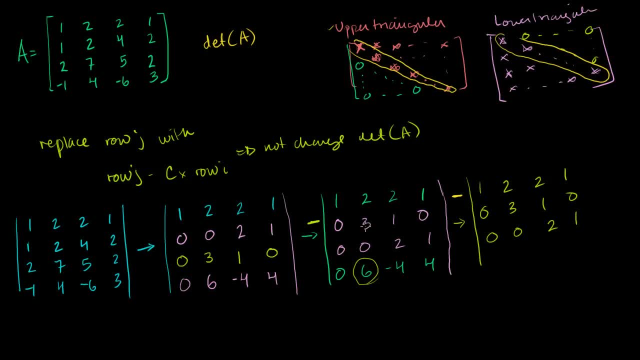 minus 3 times, or this last row minus 2 times the second row, if I want to zero it out. So 0 minus 2 times 0 is 0.. 6 minus 2 times 3 is 0.. Minus 4 minus 2 times 1 is minus 6.. 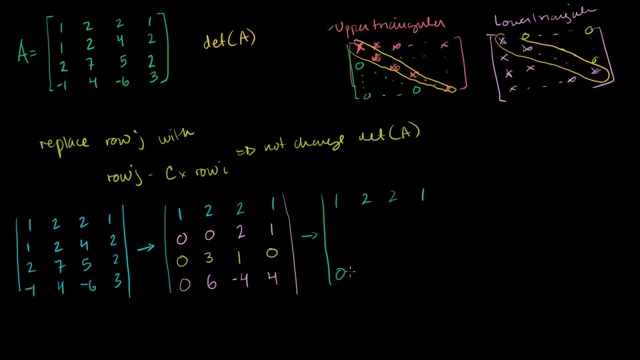 1, 2, 2, 1.. I'm going to keep the bottom row the same: 0, 0, 6, minus 4, 4.. And I'm going to swap these guys right here. So this is going to be 0, 3, 1, 0.. 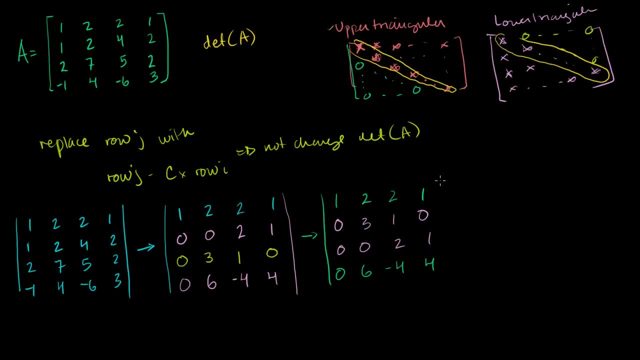 And then 0,, 0,, 2,, 1.. Now can I just swap entries like that? Well, I can, but you have to remember that when you swap entries, your resulting determinant is going to be the negative of your original determinant. 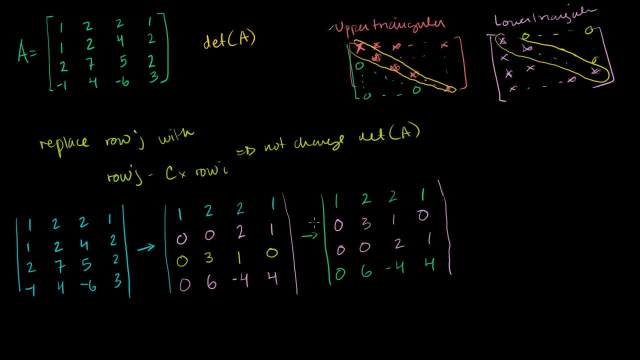 So if we swap these two guys, the determinant of this is going to be the negative of this determinant. When you swap two rows, you just flip the sign of the determinant. We saw that That was one of the first videos we did on these kind of. 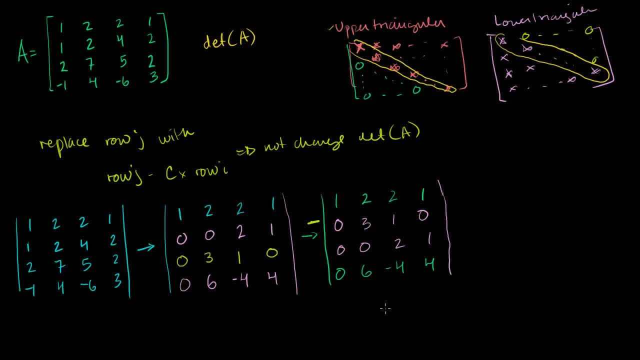 messing with the determinants. Now, what do we want to do here? To get this guy into upper triangular form. to get this in upper triangular form, it'd be nice to get this to be a 0. So to get that to be a 0,, let me keep everything else the. 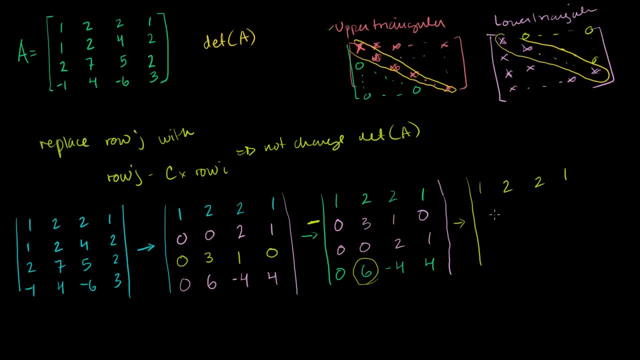 same. so I have a 1, 2, 2, 1.. I have a 0, 3, 1, 0.. The third row is 0, 0,, 2, 1.. And now this last row. let me replace it with the last row. 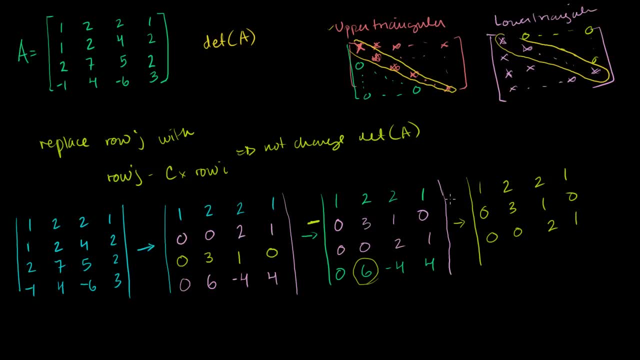 minus 3 times this row. So let me write it like this: Well, I have to carry that negative sign as well, So I'm going to replace this: This last row minus 2 times the second row. I want to 0 it out. 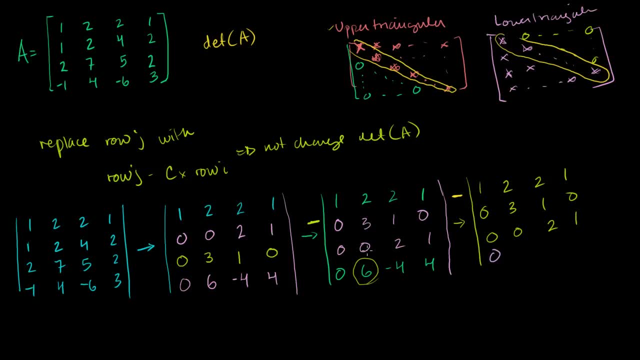 So 0 minus 2 times 0 is 0.. 6 minus 2 times 3 is 0.. Minus 4 minus 2 times 1 is minus 6.. And then 4 minus 2 times 0 is just 4.. 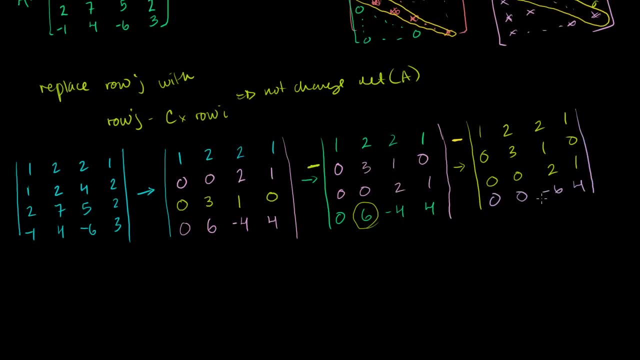 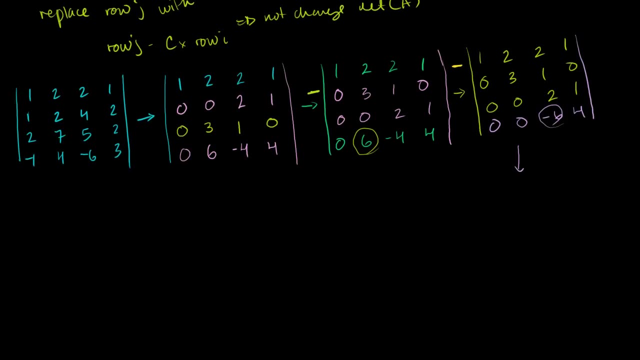 We're almost there. Now we want to 0.. What do we want to do? We want to 0 this guy out, So let's replace this one. So I'm going to keep my top three rows the same again, And let me see if I can write it a little bit neater. 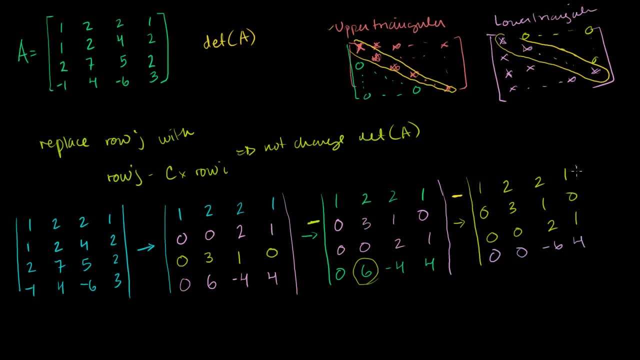 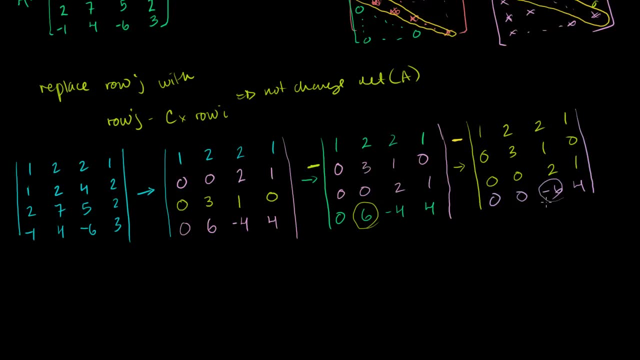 And then 4 minus 2 times 0 is just 4.. We're almost there. Now what do we want to do? We want to zero this guy out, So let's replace this one. So I'm going to keep my top three rows the same again. 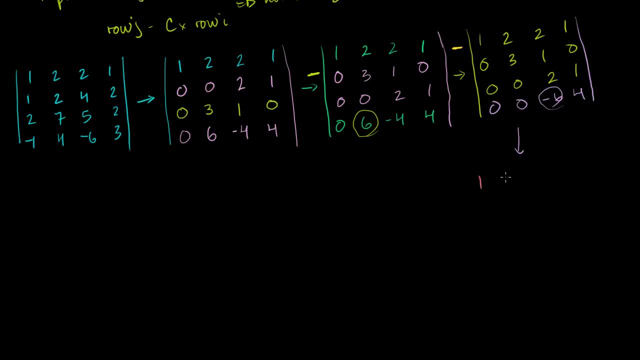 Let me see if I can write it a little bit neater. So my first row is 1, 2, 2, 1.. My second row is 0, 3, 1, 0.. Fourth row is 0, 0, 2, 1.. 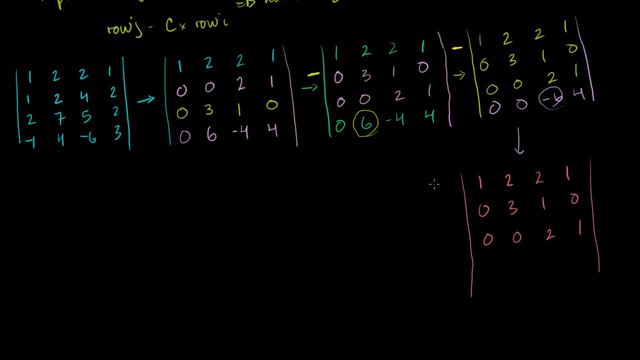 And I'm going to take the matrix. I haven't written the fourth row yet And of course, this is going to be negative of this. This is going to be the determinant of our original matrix, because we had swapped those rows. But let's replace this last row with the last row plus 3 times. 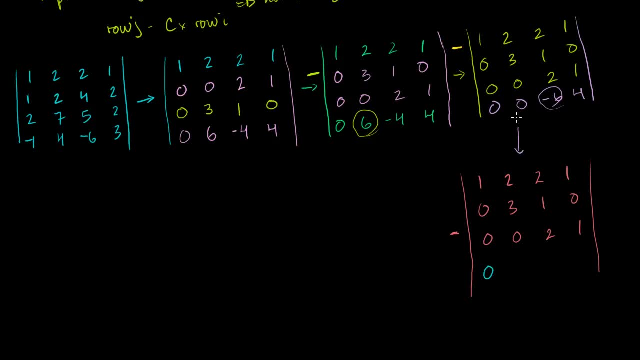 the third row. So we get: 0 plus 3 times 0 is 0.. 0 plus 3 times 0 is 0.. Minus 6 plus 3 times 2 is 0.. 4 plus 3 times 1 is 7.. 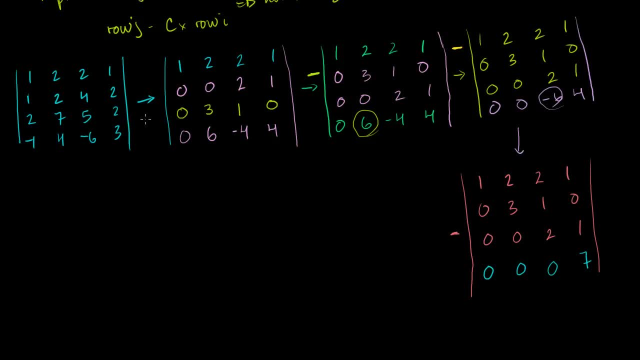 And just like that, we have a determinant of a matrix in upper triangular form. So this is going to be equal to the product of these guys. So this is going to be equal to- can't forget- our negative sign. let's throw our negative sign out there and put a. 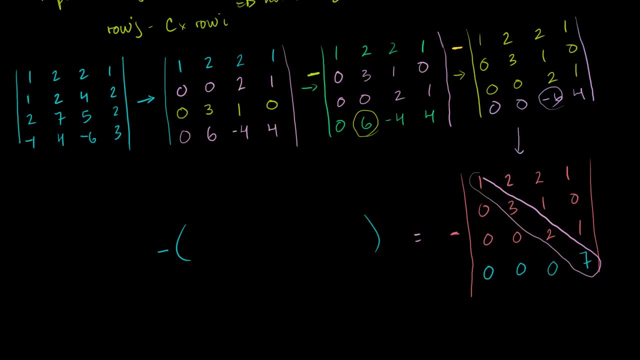 parentheses, just like that. This is going to be the product of that diagonal entry: 1 times 3 times 3 times 2 times 7, which is 6 times 7,, which is 42. So the determinant of this matrix is minus 42.. 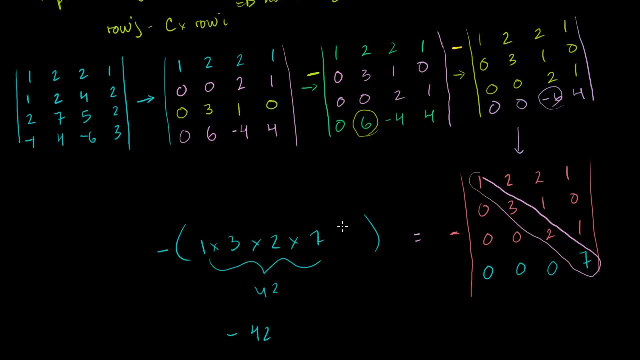 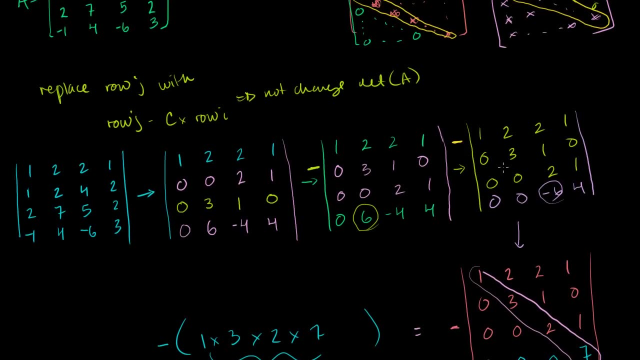 OK, OK, OK, OK, Which was pretty fast. This was a pretty fast shortcut And it actually turns out. it tends to be computationally more efficient to use these takeaways to put things into upper triangular form first, And then you know if you do swaps. you have to remember to. 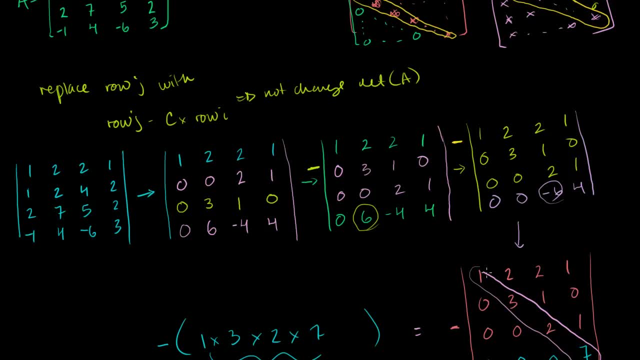 make the determinant negative And then just multiply down the diagonal, And we did that. there We got the determinant as being minus 42..